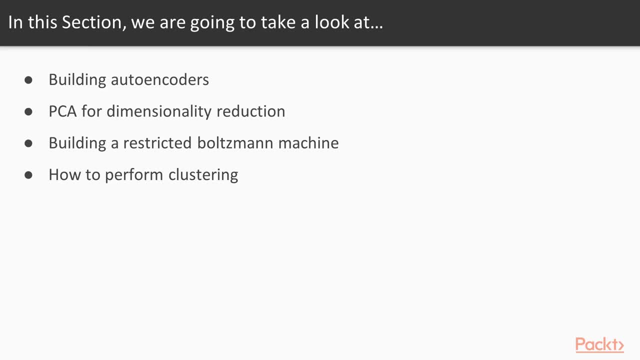 use them to extract features from a dataset. We will use the Higgs boson dataset. In the second video we talk about PCA, or principal component analysis, a well-known technique for dimensionality reduction. We will see how to implement this technique using TensorFlow In the third video. 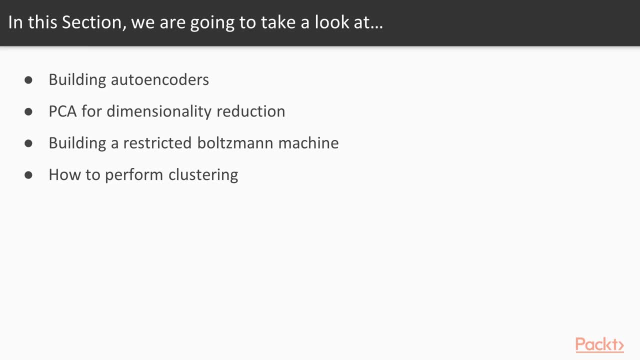 we talk about these special types of neural networks called restricted Boltzmann machines, and we use them to represent images using less information. In the fourth and final video of this section, we will talk about clustering, a well-known unsupervised learning technique, And in particular, we will see how to use TensorFlow to perform. 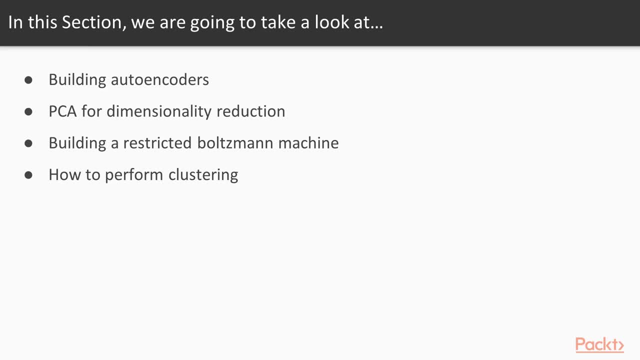 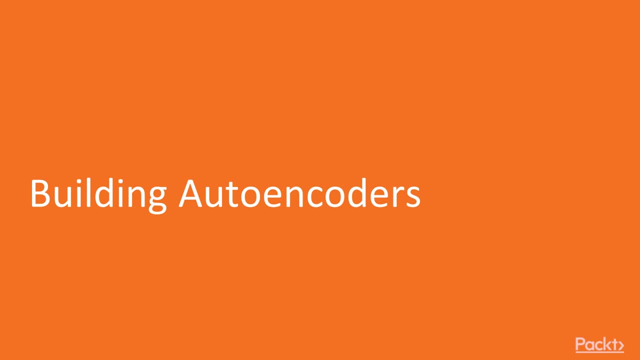 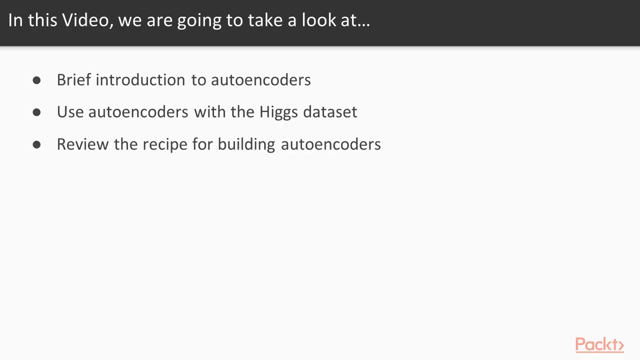 k-means clustering. So this is the plan for this section. Let's begin. This is the first video of this section, and here we talk about autoencoders and how to build them using TensorFlow. So this is the plan for this video. First, we will give a brief. 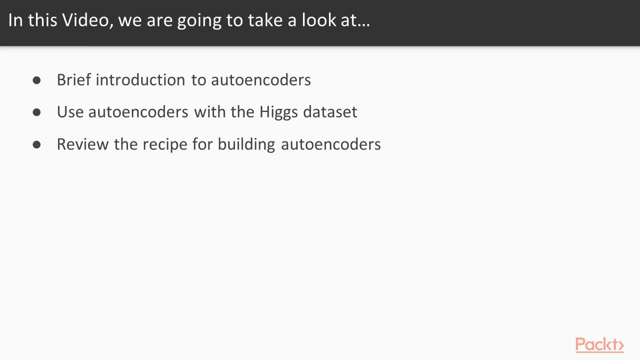 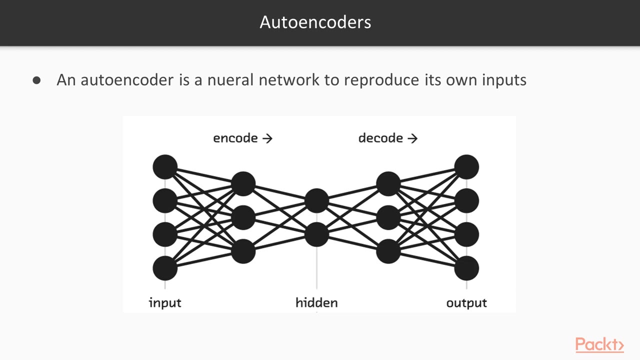 introduction to how to use TensorFlow to perform k-means clustering. Then we will use autoencoders with the Higgs boson dataset And finally we will review the recipe for building autoencoders. Okay, what is an autoencoder? An autoencoder is a neural network built to reproduce its 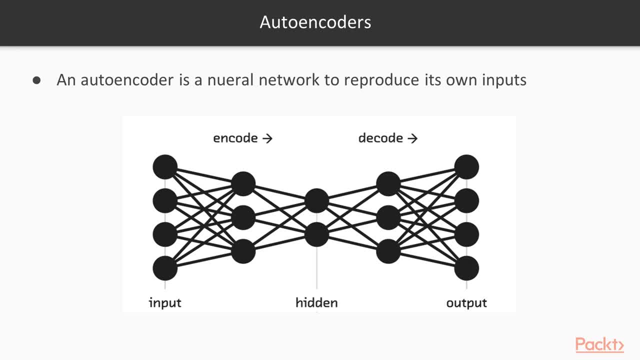 own inputs. Remember, we are dealing here with unsupervised learning, so we don't have targets, And in this case, what we want to do with these autoencoders is to build them using TensorFlow. So what we want to do with these autoencoders is to build a neural network. 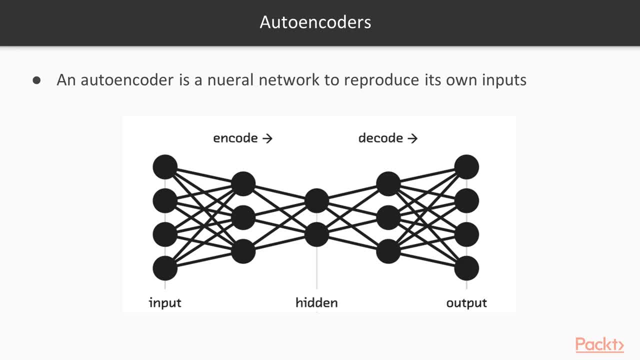 capable of reproducing as best as it can its own inputs. So you can see here a simplified example of an autoencoder. We have some inputs. then we pass these inputs through a set of hidden layers and the first step is called encode, And then one of the restrictions that we have in autoencoders. 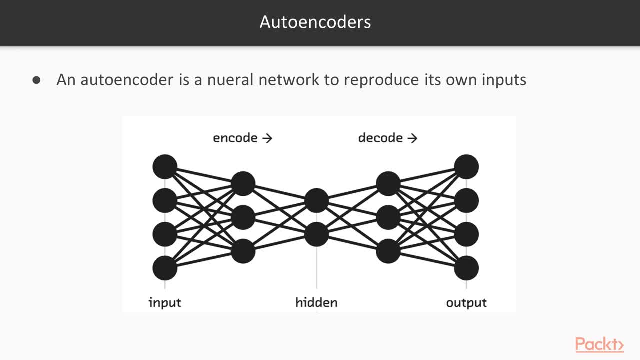 is that we use lower dimensionality here in the hidden layers, And then with using this lower dimensionality we try to represent the same input here. So we try to make this output as close as the input. So that is how autoencoders work. 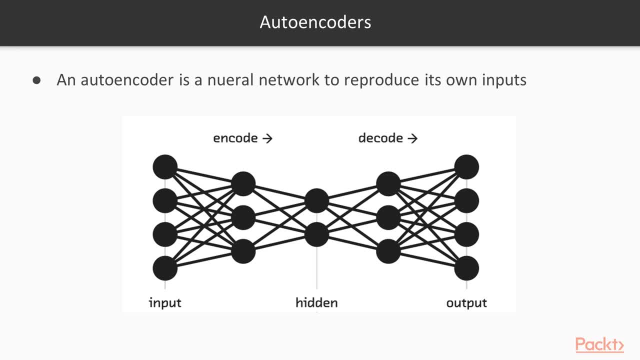 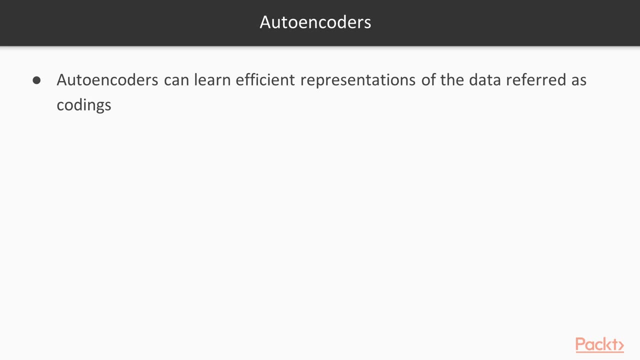 And the goal of this process is to produce some what are called codings that contain an efficient way of containing the information present in the inputs, So autoencoder can learn efficient representations of the data referred as codings. The codings is what we want. 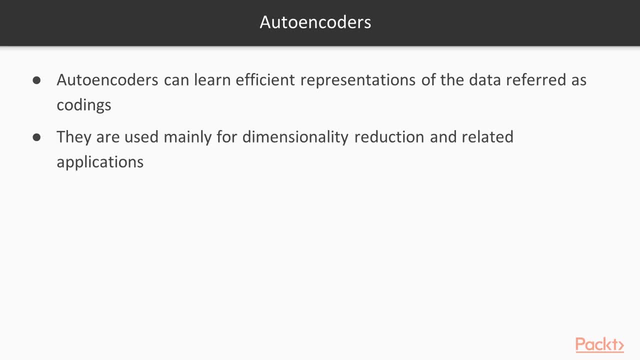 from the autoencoder. as we will see in the example, They are used mainly for dimensionality reduction and related applications, and they can be also used to extract new features from data, and that's how we are going to use the autoencoder in our example. Another use of autoencoders is to: 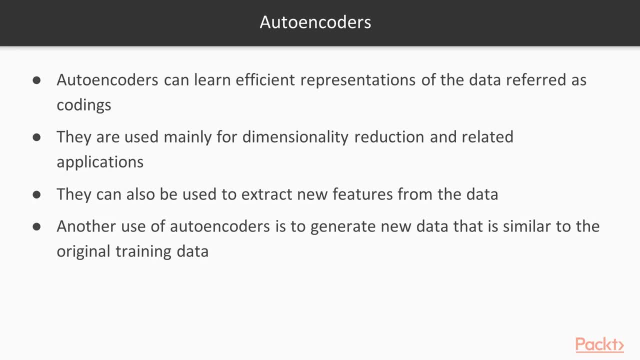 generate new data that is similar to the original training data. Sometimes we need to expand the data that we have available for training, and autoencoders can be a nice tool for doing that. One interpretation of the codings is as features detectors, So the codings can be thought of as 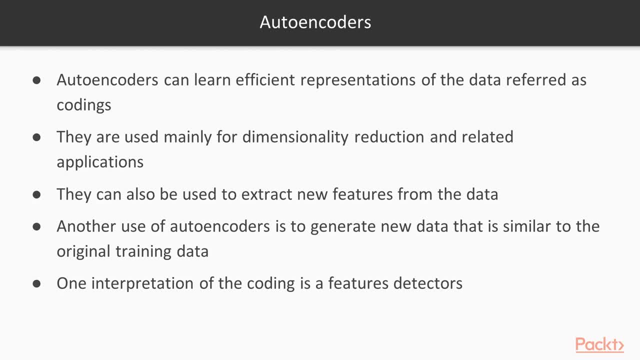 different features that may help us solving the problem that we have, and autoencoders are very, very similar to multi-level perceptions, which are the multi-level perceptions, which are the multi-level perceptions, which are the types of neural networks that we have been using in this course. 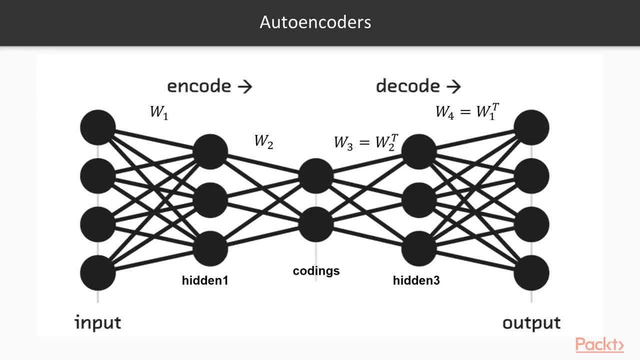 Okay, so here we have the same picture that I showed you before, but this is a representation of the implementation of the autoencoder that we will do in the example. So here we have some inputs, and then we pass these inputs to a hidden layer, and this hidden layer has its own weights. 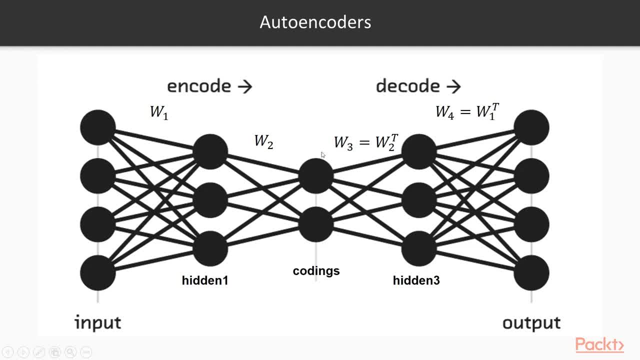 and then we pass this to another hidden layer and notice that this hidden layer has lower dimension than the original input. So these are the codings. the second hidden layer in this case are the codings. This hidden layer also has its own weights. Now we pass the resulting values from this layer to a third hidden layer. 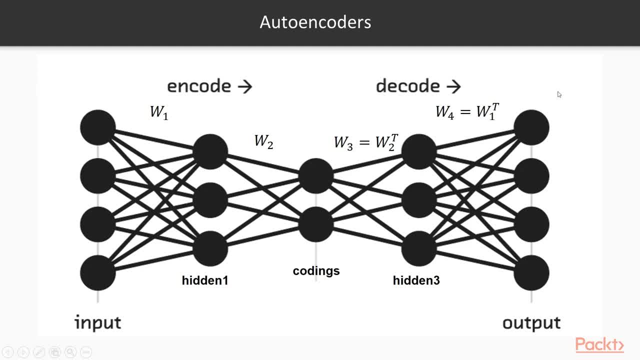 and then we pass this to the output, and this is the output layer, and the output, of course, has the same dimensionality as the input, because we want to make the output, the output, as close as possible to the input. Now an additional restriction that we will impose in our 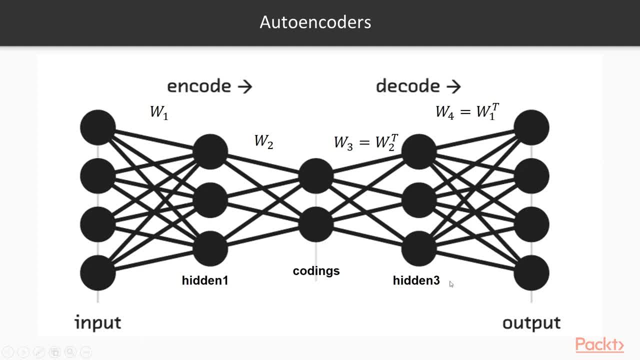 the output as close as possible to the input. Now, an additional restriction that we will impose in our network, in this autoencoder, is that the weight for the third hidden layer must be the same. The weights must be the same as the weights that we had in the second hidden layer. So, as you, 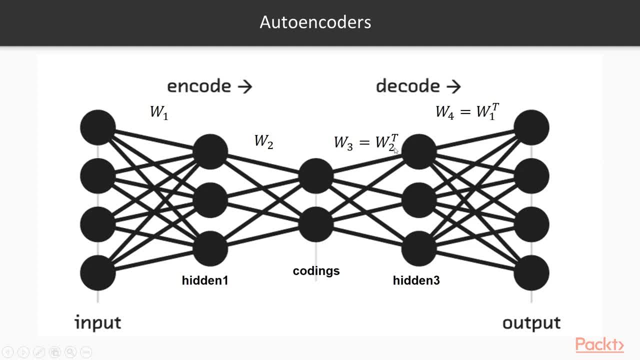 can see, here we have the same weight, we have the same weight matrix. However, it is transposed because, for example, here we are going from three dimensions to two dimensions, and since here we are are going from two dimensions to three dimensions, again we have to transpose this. the same happens. 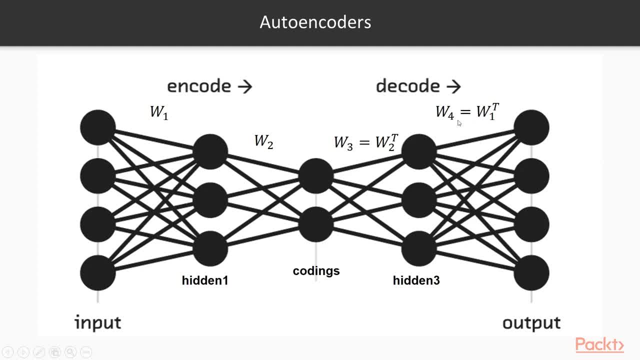 here with the weights for the last layer. we will use the same weights as we have here in the first hidden layer, so the same thing. we have to transpose them and this is an additional restriction that we impose in our network so the network can learn the most efficient representation from the inputs. 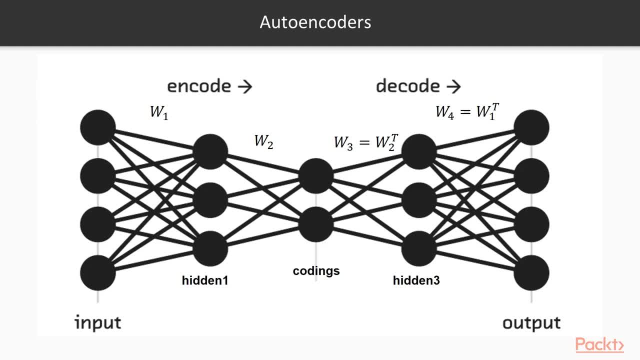 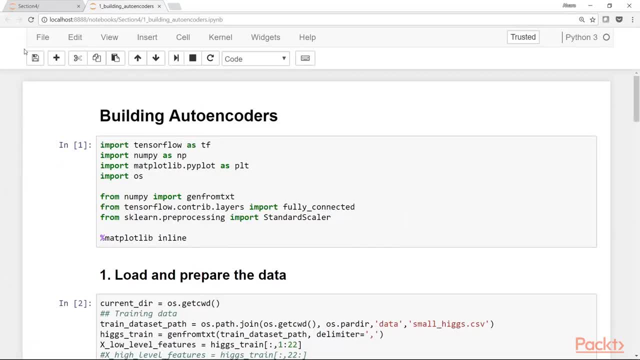 okay, now that we have the intuition about what out on coders do, let's go and see the example. okay, this is the jupiter notebook we will use for this example, and the task that we are going to do is to take some of the features that we have in our original higgs boson dataset and try to get 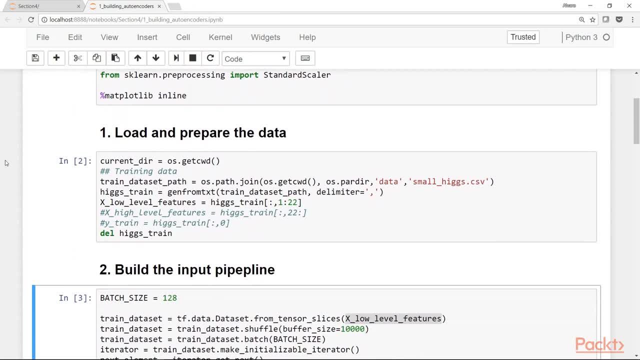 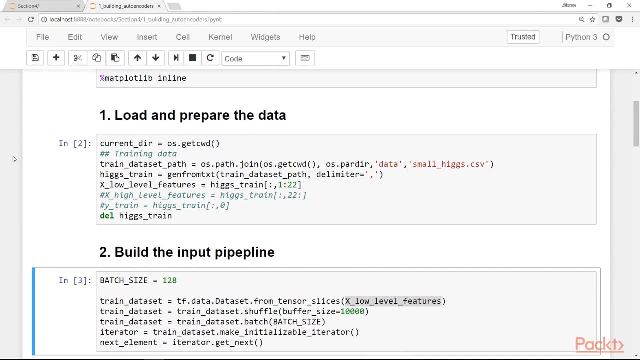 new features from those features. so, as always, the first step is to load and prepare the data. since you parents are doing here some unsupervised learning, we only need the matrix containing the features, so we don't need the targeting in this case. now, remember when i introduced this data set, i told you that we 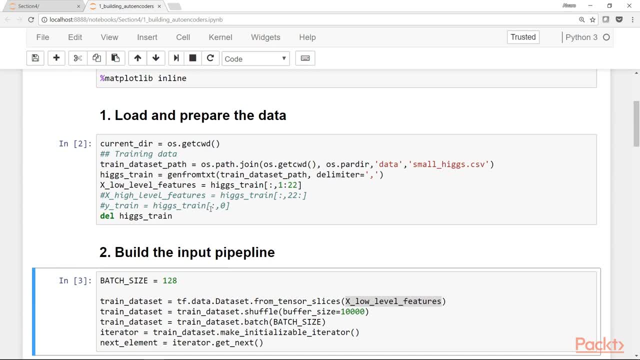 have two types of features here. we have 21 that are considered low level features and we have another seven that are considered a high level feature. so what we are going to do here is to use these low level features and we will try to get some transformation of these features. some: 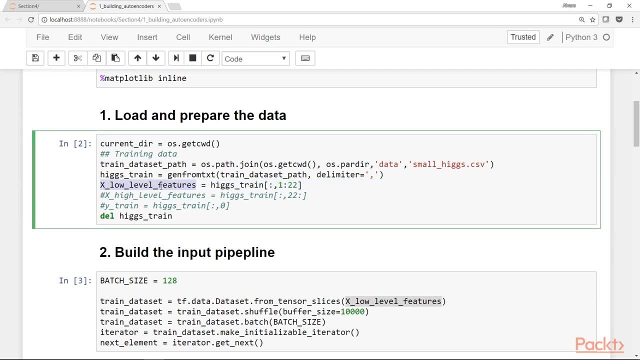 efficient representation of these 21 features in four new features. so these four features may be helpful for doing other tasks, like detecting if there is a signal for the higgs boson. so this is the task that we are going to do in this example. so this is the first step. second step is to build. 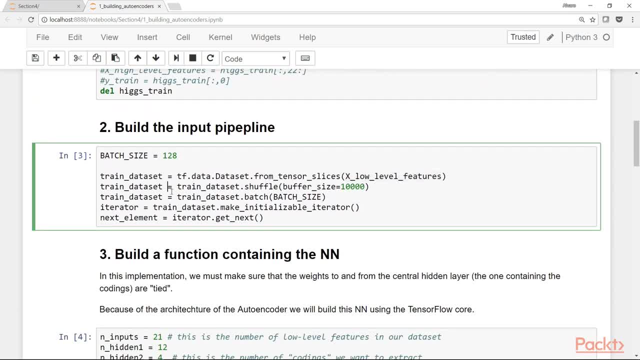 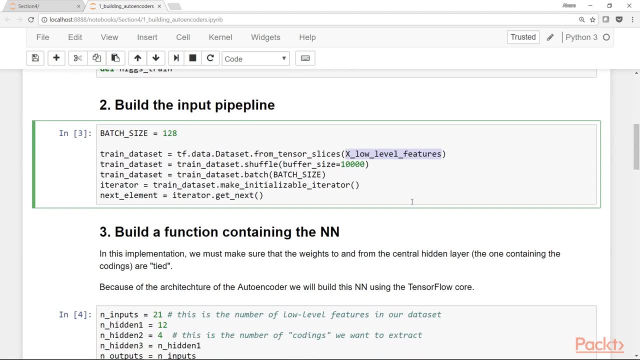 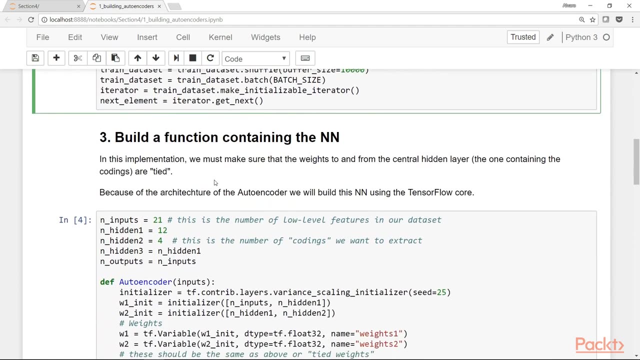 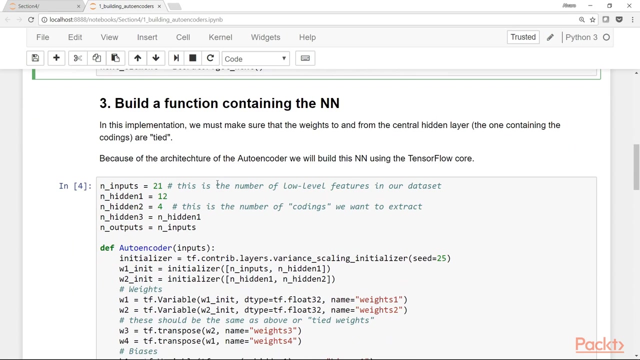 the input pipeline, and we have seen this code before. in this case, we will use again the dataset api and we will use only the matrix containing the low level features. so this is the second step. the third step is to build a function containing the neural network, and we will see how to implement the network that i showed you. 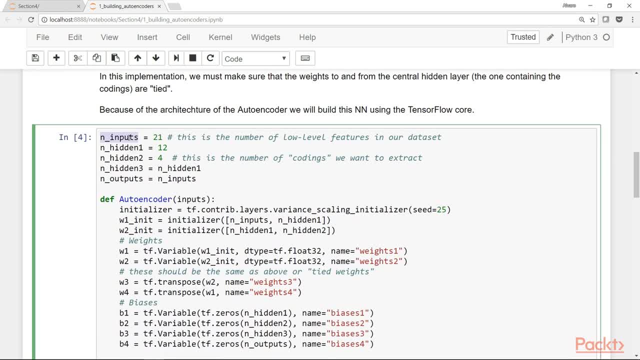 back in the presentation. so first, this is the number of inputs that we have. so we have 21 features that we would like to use to get these new features. so 21 features. we want to capture as much information as we can from these 21 features, the first hidden layer in our network. we 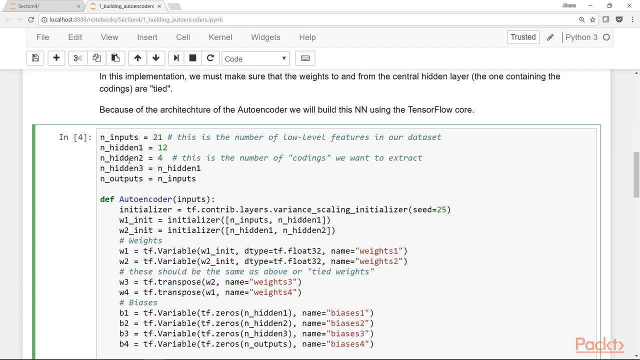 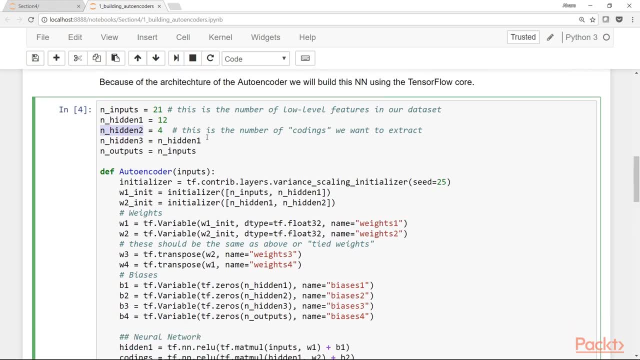 have 12 neurons and the second hidden layer will have four. so this is the number of codings that we want to extract. so we want four new features. in this case, this is the corresponds to the middle of the network. so we will extract the values from this layer and then 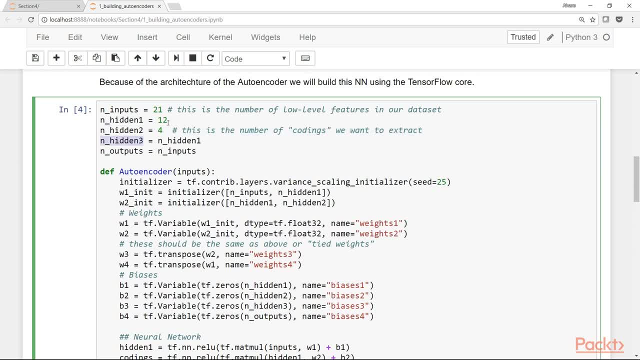 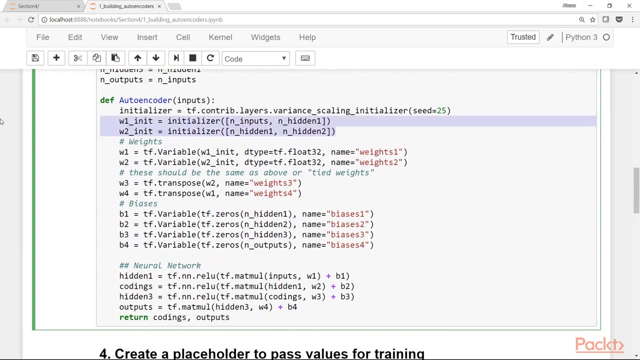 in the, the third hidden layer, we'll have again 12 neurons and the outputs. the number of outputs that we want is the number of inputs, because we would like to reproduce the inputs as well as we can. okay, so this is the function containing the auto encoder. what these three lines do is just to: 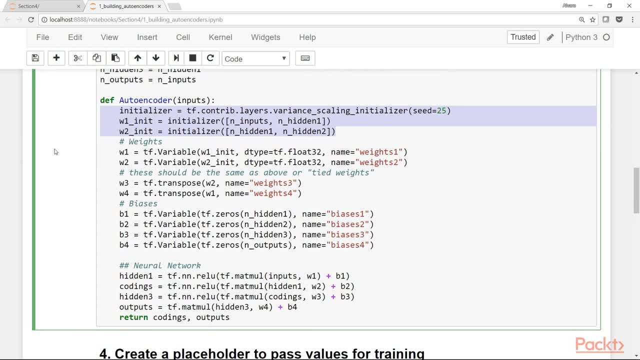 initialize the weights for the function that we want to use to get the output that we want to use. so we have the first two layers in our network. so these are the weights for the first hidden layer and these are the weights for the second hidden layer. as i told you in the presentation, the 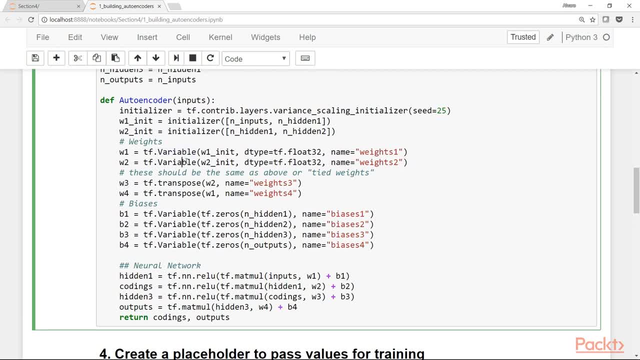 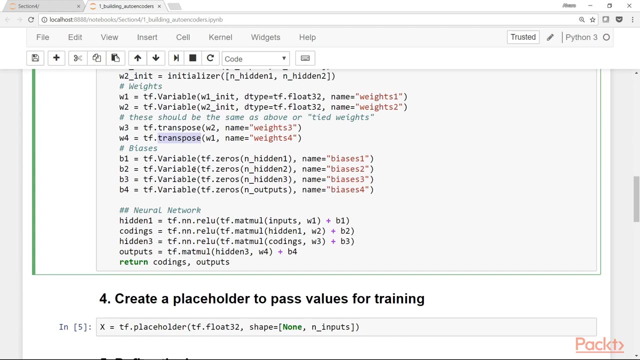 weights for the third and for the fourth hidden layer are the same weights that we used here. that's why we have the same here. we are just transposing the the corresponding values. okay, now we have the biases for every layer in our network. we will just initialize the biases with zeros and here we have the actual neural network. 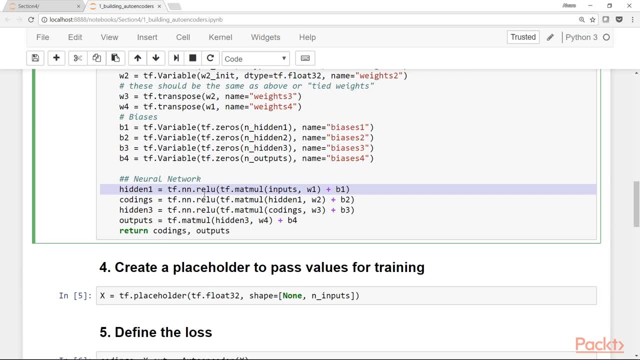 so the first hidden layer, just this is basically the operation that gives us a hidden layer. so applying the relu to the matrix: multiplication of the inputs times the weights plus the bias. okay, and this is the middle of the network. this is the second hidden layer, but we called it here. 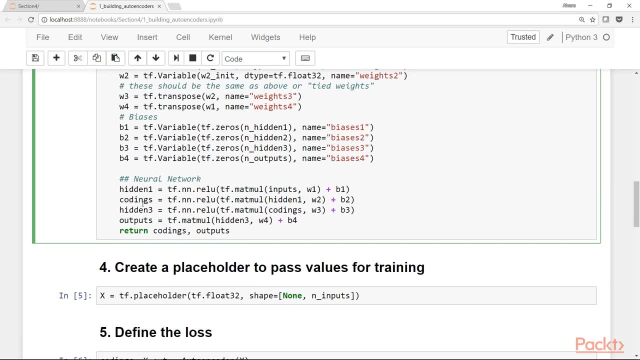 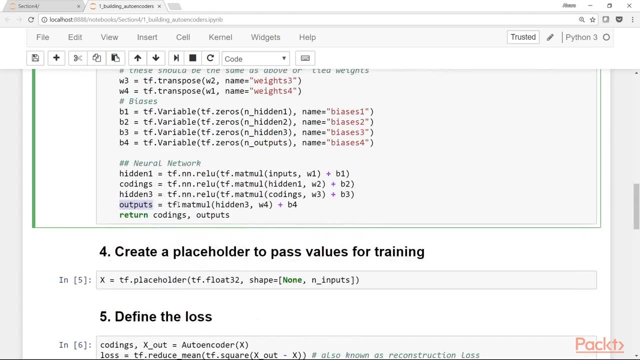 the conings- this is what we want to extract from this network. and finally, in the outputs, this is the output layer. okay, so what we are going to return from this function are the conings and the outputs. okay, this is the third step and we just implemented. 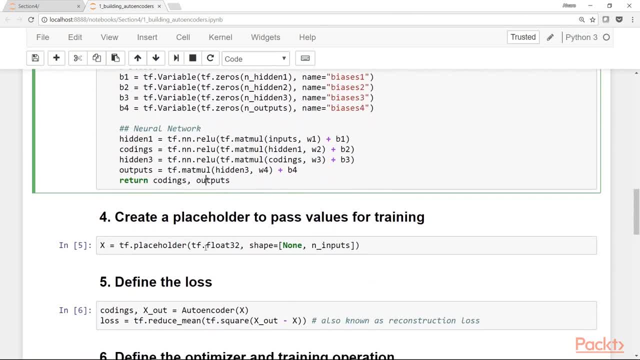 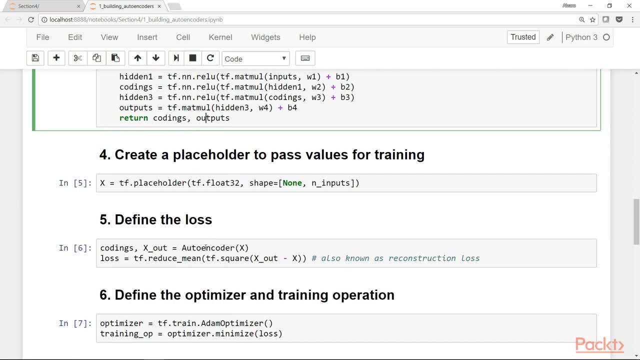 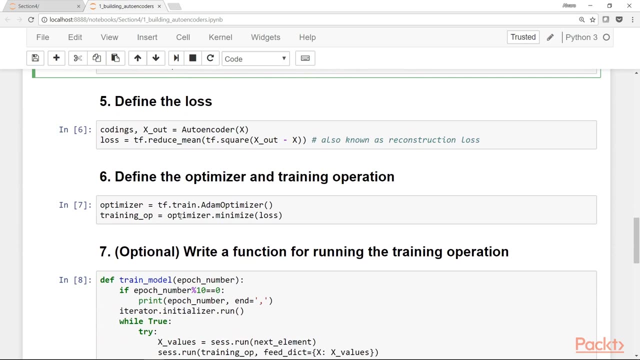 a network based on the description that i gave before during the presentation. now, step number four is to create a placeholder to pass the values for training- and in this case we only need a placeholder for x, because this is unsupervised learning- and step number five is to define the loss. 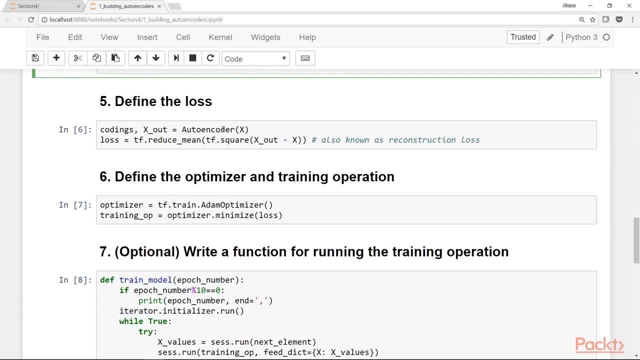 so we want two things from this function: from the autoencoders, we will get the x, the output, the representation of the original input, and what we want is to reduce the distance between the square distance between the output and the original input of the network. this what you have. 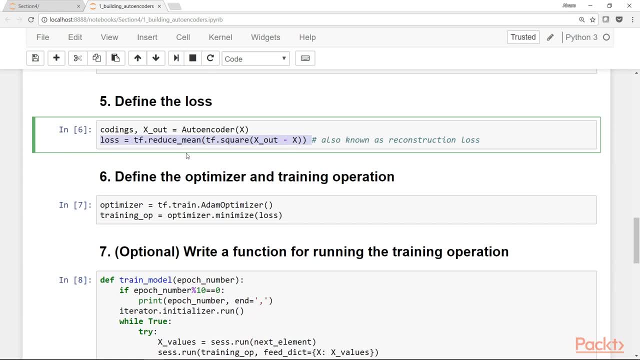 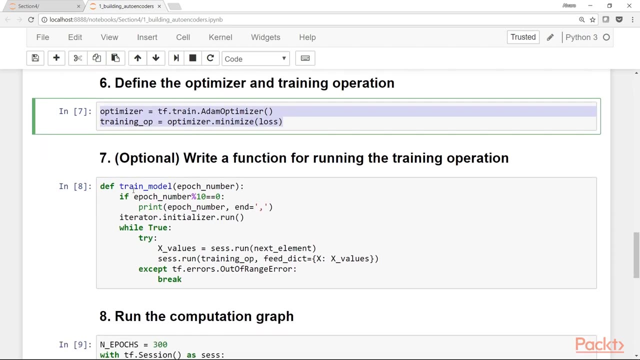 here we take the mean. we are essentially calculating the mean squared error here. this is also known as the reconstruction loss. okay, so this is the loss that we will minimize, and we will minimize it using an optimizer. so we know this operation very well. now step seven is to well. this is, as always, this is an optional step, but this 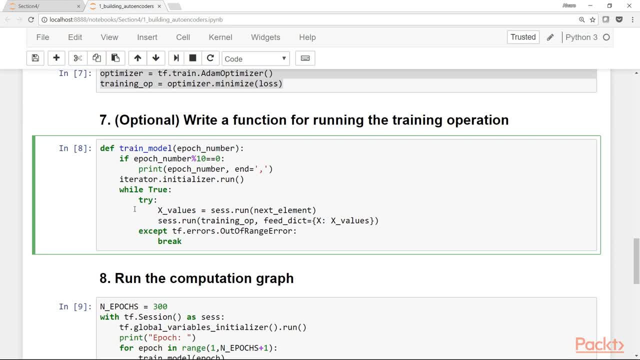 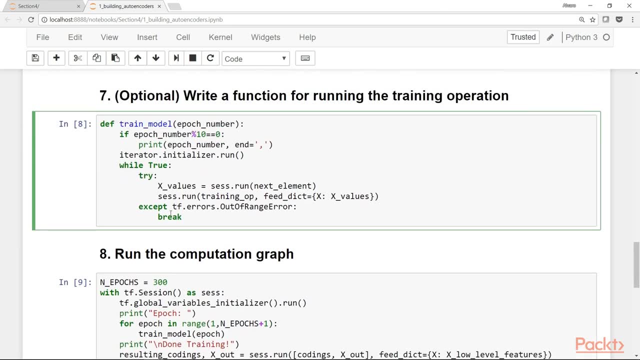 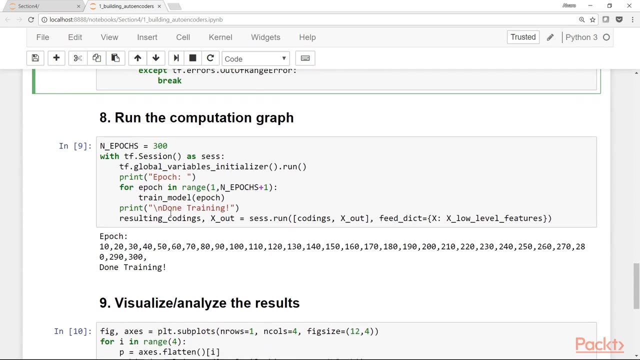 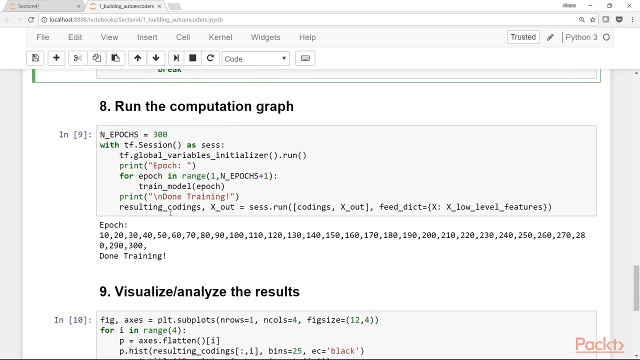 will make your code more readable. we write a function for running the training operation. so we've seen this code before, or a version of this code before. and finally, in step eight is to run the computational graph. okay, so now, once the network has been trained, we have our optimal values for our weights and we can 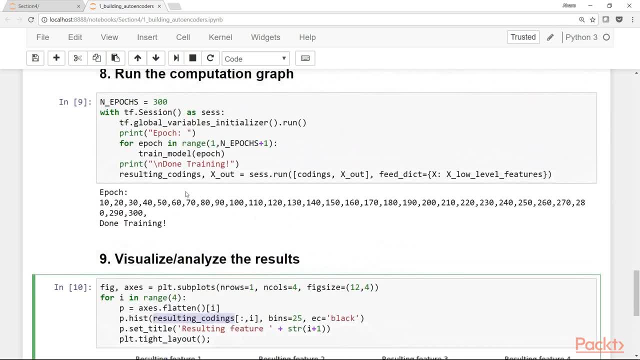 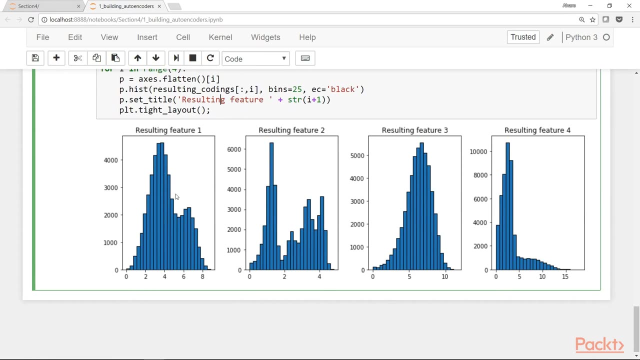 get our resulting coins here. so we got the resulting coding here by running these two nodes from the computational graph. so we have here the resulting coins and this is how these new features look like. so i just named them resulting feature and so we have these four new features contain an efficient representation. 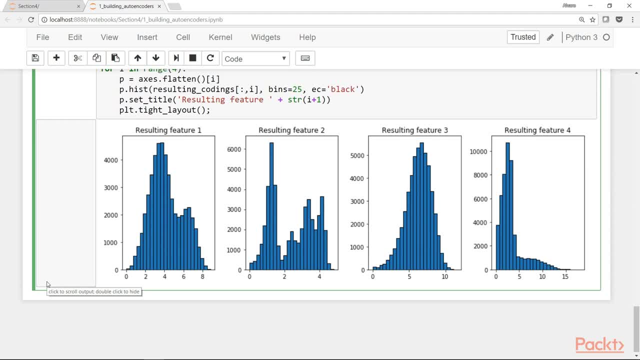 of the 21 features that we used as input for this network. so now these could be used, as i said before, for example, to try to detect in a better way the signal that can lead to the higgs boson, but we don't know if this will actually. 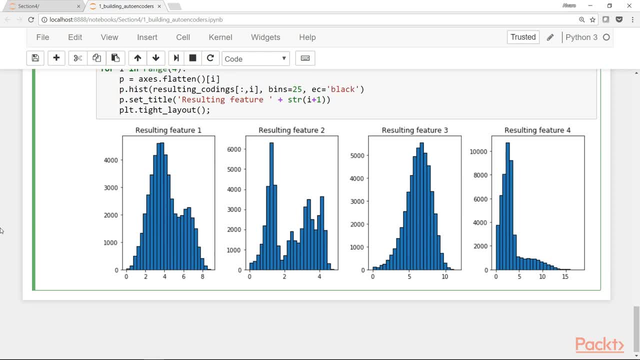 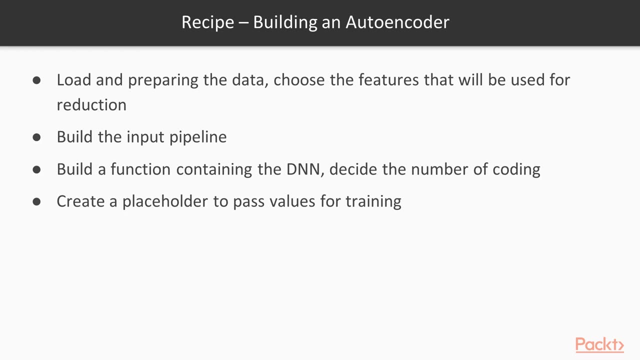 so that is another subject, but at least we have here four new features that represent efficiently the information contained in the original 21 low level features. okay, great. so this is a little review of the recipe we saw in the notebook: how to build and how to encoder using tensorflow. the first, as always, the first step is to load and prepare the data. 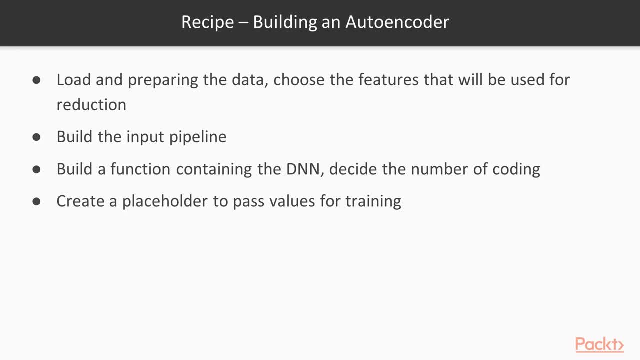 the second step will be to build the input pipeline. the third step is to build a function containing the neural network, and here you decide how many features you want from your autoencoder. number four is to create a placeholder to pass the values for training, and here we pass just the x values, the x matrix. uh, that contains the original features. 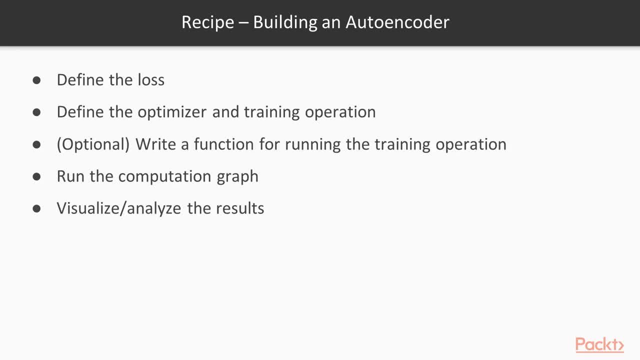 uh, step number five is to define the loss. step number six is to define the optimizer, and training operation in step seven is optional, but we write a function for running the training operation. Step number eight is to run the computational graph and then you visualize it or analyze. 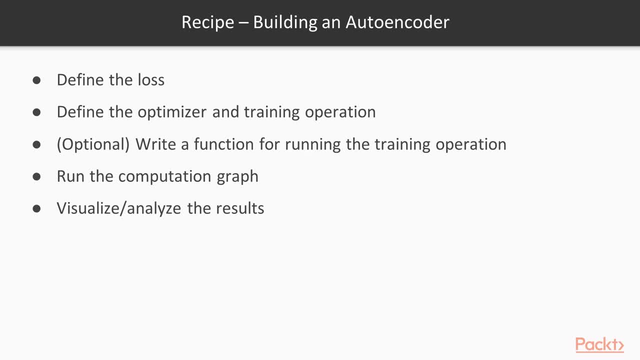 the results Now. as you can see, this recipe looks very, very familiar. It looks almost exactly as creating a deep neural network, because in the end, an auto encoder is just a special kind of neural network, So you only have additional restrictions, but it's in a sense a neural network. 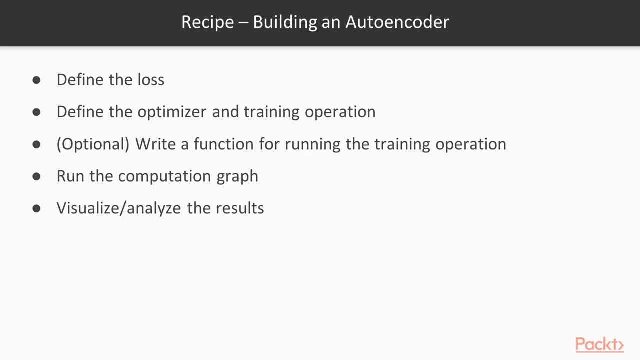 Okay, In this video we learn how to build an auto encoder to get features that are an efficient lower dimension representation of the original data.